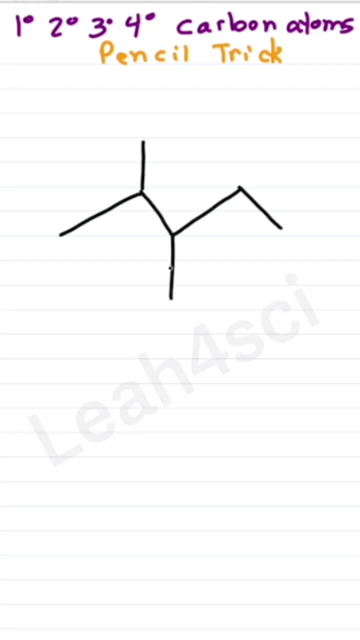 Can you classify every carbon atom as primary, secondary, tertiary or quaternary? Let's use the pencil trick to simplify. For the pencil trick, you put your pencil down on carbon and ask: how many lines can I draw from here to another carbon? I got four, making it a quaternary. 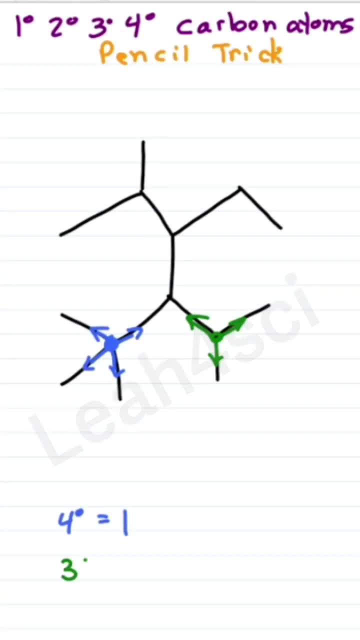 carbon. What about this one? I got three, making it a tertiary carbon. But doesn't this one also have three? On this carbon, I can draw two lines making it secondary. But wait, I have another carbon that has three lines and another one with three lines. That's two more tertiary carbons. 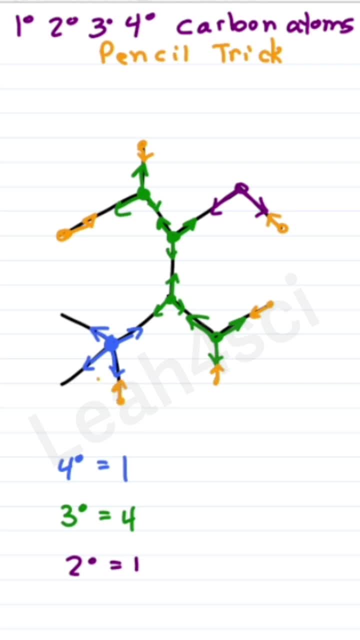 And finally, if I can draw just one line, that's a primary carbon for a total of eight. 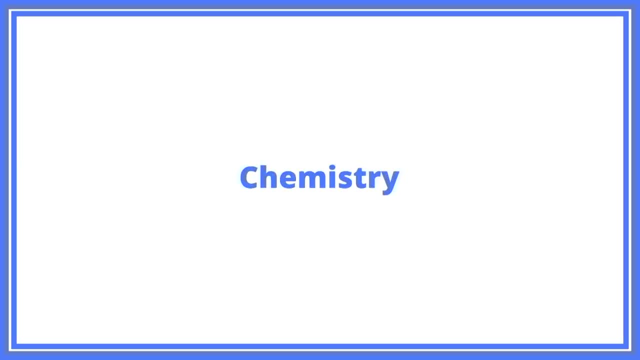 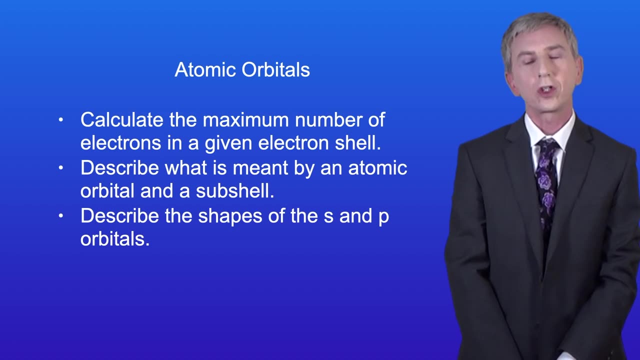 Hi and welcome back to Free Science Lessons. By the end of this video, you should be able to calculate the maximum number of electrons in a given electron shell. You should then be able to describe what's meant by an atomic orbital in a subshell And finally, you should 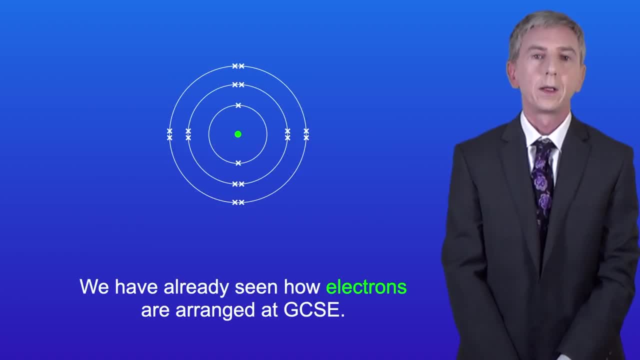 be able to describe the shapes of the s and p orbitals. Now we've already seen how electrons are arranged. at GCSE We saw that electrons exist in electron shells. We saw that the first shell can hold up to 2 electrons and the second 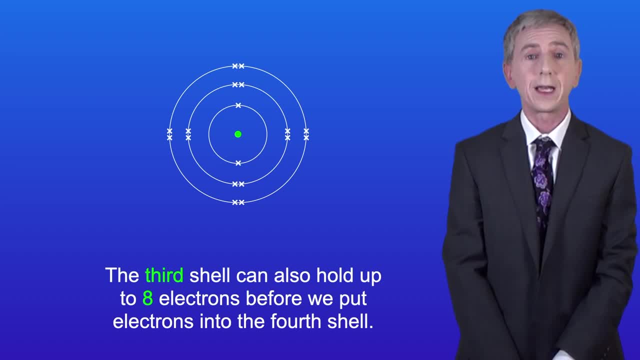 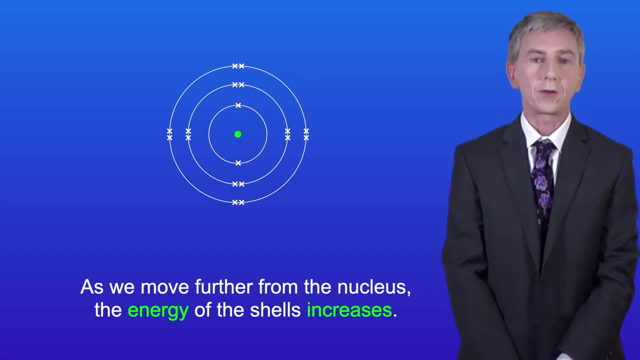 shell can hold up to 8.. The third shell can also hold up to 8 electrons. before we put electrons into the fourth shell, And as we move further from the nucleus, the energy of the shells increases. Now that's a relatively simple description of electron shells, but at A-level we need: 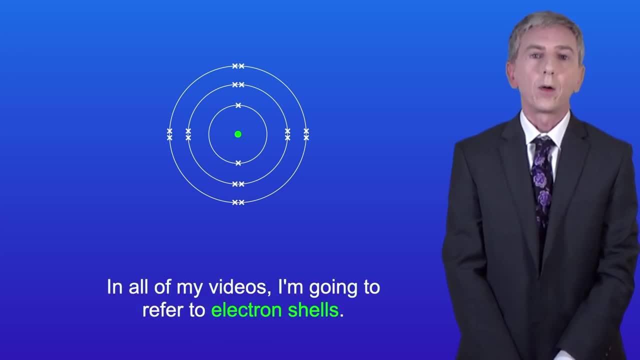 to go into a lot more detail, So let's get started Now. I should point out that in all of my videos, I'm going to refer to electron shells. However, the AQA example is a little bit different. The AQA example is an electron shell that. 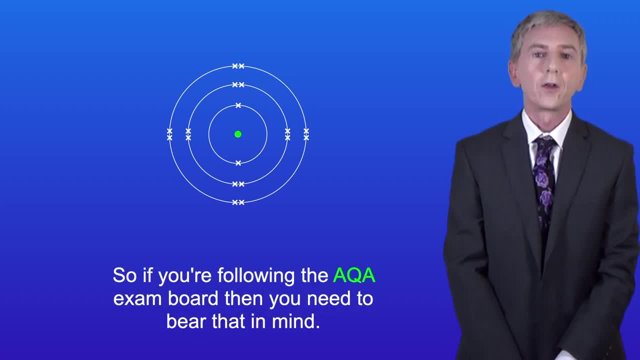 has two cells and two electrons. In fact, it has two cells and two electrons. Now, the AQA example in the AQA example board refers to electron shells as main energy levels. So if you're following the AQA example board, then you need to bear that in mind.